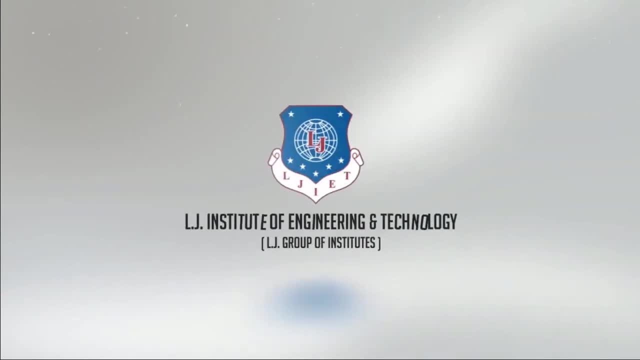 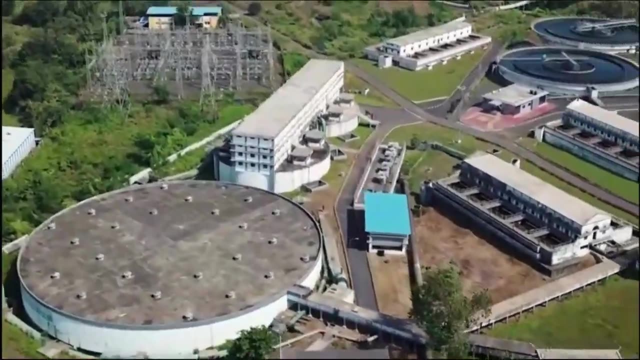 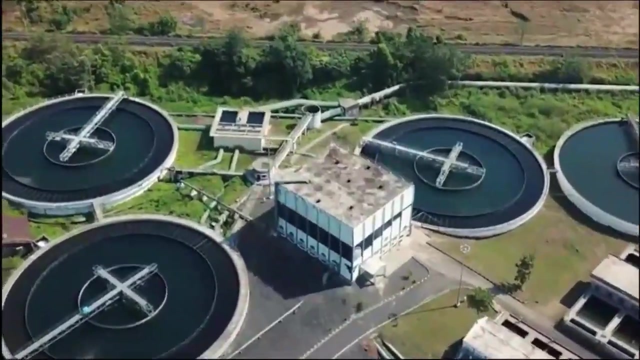 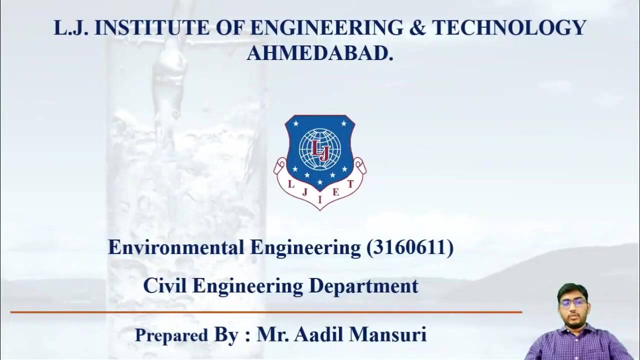 Welcome back students to the video lecture series. I am Adil Mansoori from civil engineering department of engineering institute of engineering and technology. So, my dear students, in the previous video we have discussed regarding the house drainage right: what are the different principles of house drainage and what are the different appurtenances, or what are the different? 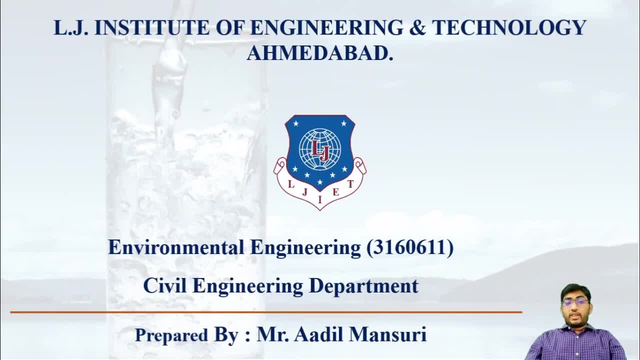 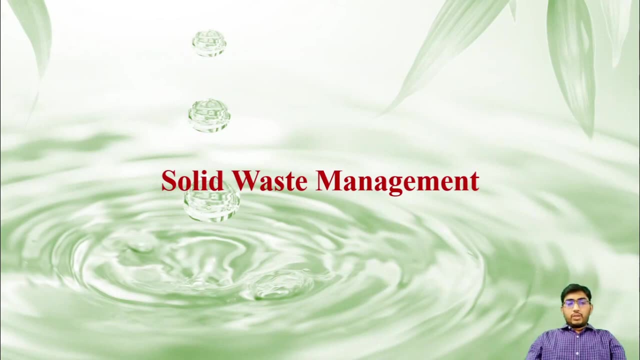 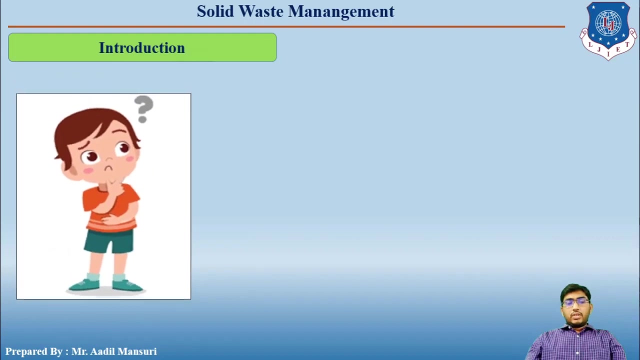 kinds of sanitary fittings that are used in the house drainage system. Okay, so now we are going to start with the next topic, that is, the solid waste management. Okay, so let us start with today's session. Let me begin with the introduction. First, let me ask you one question: What is the 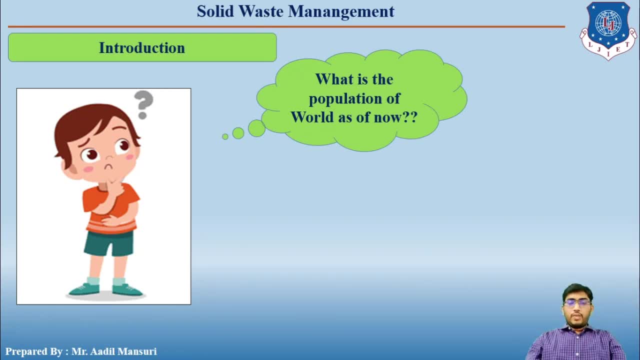 population of world as of now. Okay, so a rough estimate is there that it should be approximately 150 crore people right Now. next question I would like to ask is: what was the population of India as per 2011 census? Okay, so the answer is 121 crore people. Okay, now, do you know that, out of this 121? 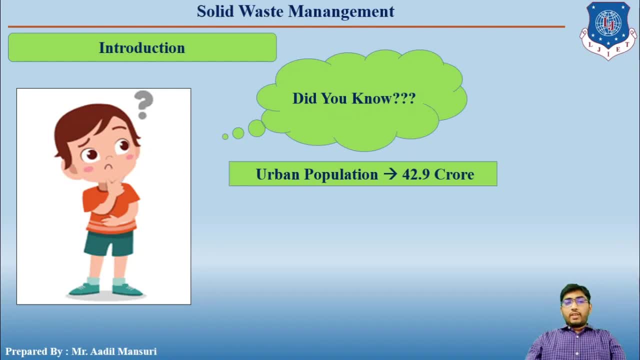 crore people. 42.9 crore people live in India. So what is the population of India as per 2011 census? In urban area, Okay, and these people create 62 million tons of garbage per year, right Out of which 5.6. 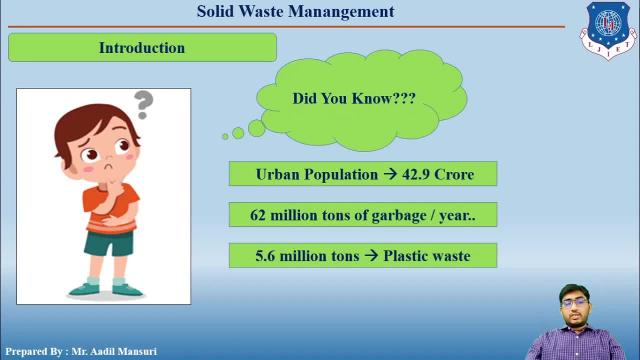 million tons of garbage is including plastic waste. 0.17 million tons includes biomedical waste. Okay, then, what is the population of India as per 2011 census? Okay, so the answer is 121 crore people. Okay, so, 7.9 million tons includes hazardous waste. Okay, and 1.5 million ton includes e-waste, But the 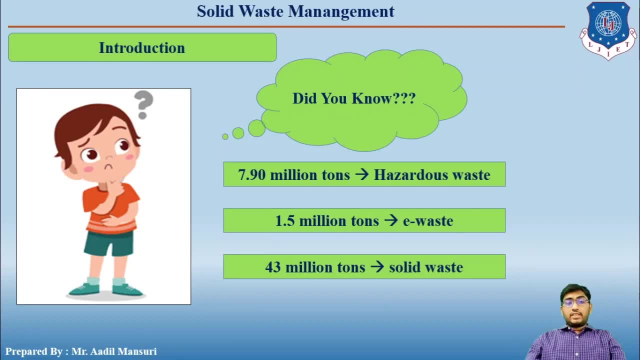 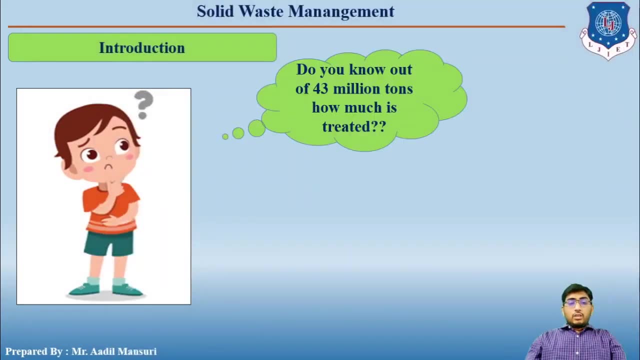 maximum is 43 million tons, and that is solid waste generation. Okay, so do you know how this 43 million tons of solid waste waste treated? so only 22 to 28 percent of the waste, that is, approximately 11.9 million tons, is treated, whereas rest 31 million tons is dumped on the landfill. 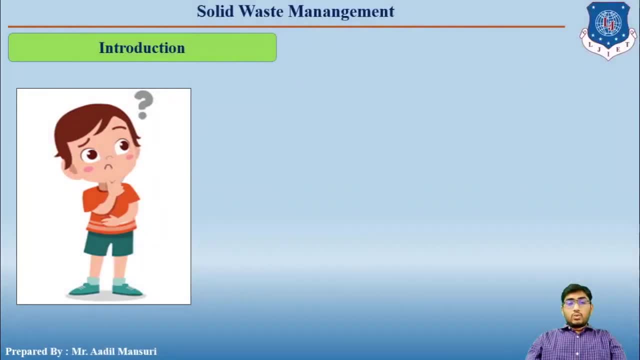 sites. okay, so which is the largest landfill site in India? do you know? the answer is Ghazipur, which is located in Delhi. it has 70 acres of land and, on a daily basis, 3,000 metric tons of solid waste is dumped on this particular. 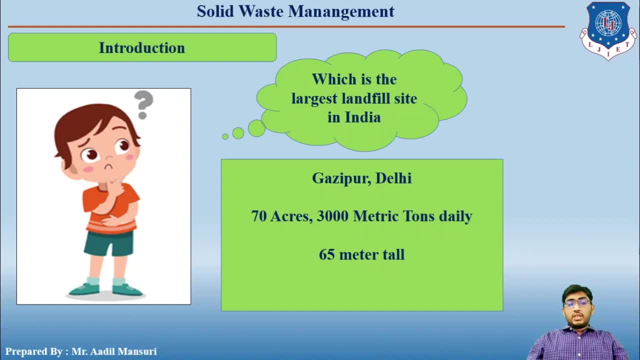 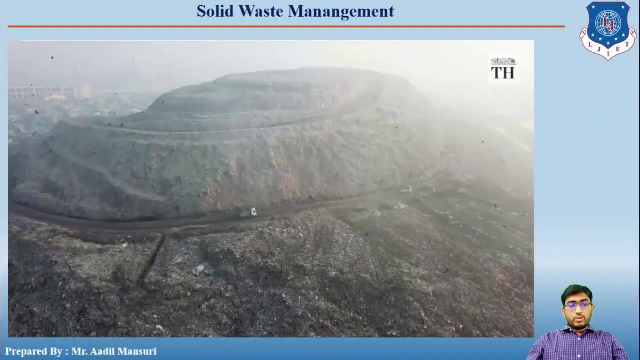 landfill site. okay, this is 65 meters tall and it it was already overshot by 15 feet in 2002. let me show you the picture so that you will get the clarity that how this Ghazipur landfill site looks like. okay, so moving forward. now, coming to the 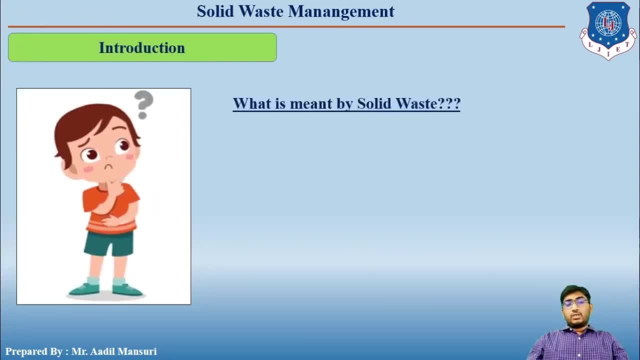 main topic: what is meant by solid waste? so solid wastes are the ways which are created by humans and차� roasted it, or animal activities that are normally solid and that are discarded as useless or unwanted- okay, that we don't have to use it again. and those ways are unwanted, right, usually the term refuse. 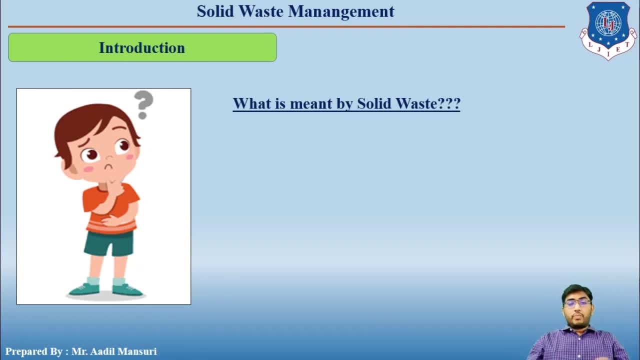 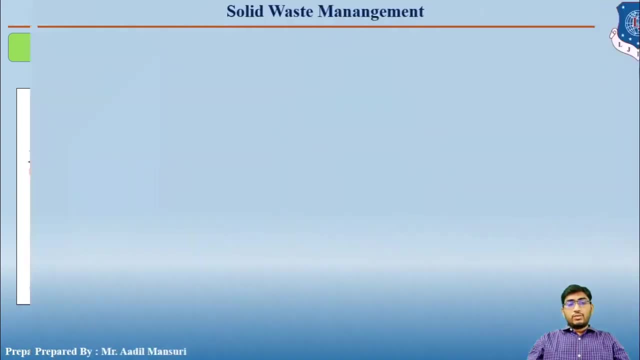 is often used in place of solid waste. okay, so let us now discuss regarding some terminologies. so the first one is the garbage. so what do we mean by garbage? so it is the waste which is coming out of kitchen and which is organic in nature and it decomposes quickly. if i talk about its density, it's usually: 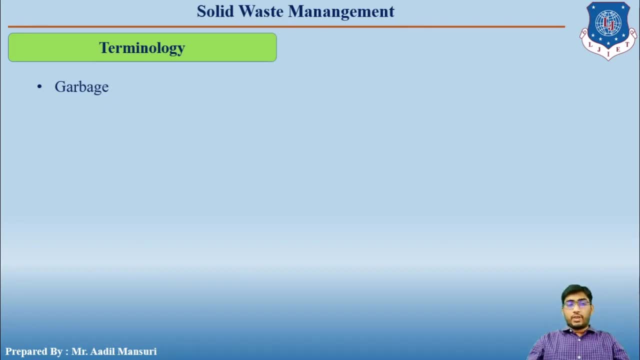 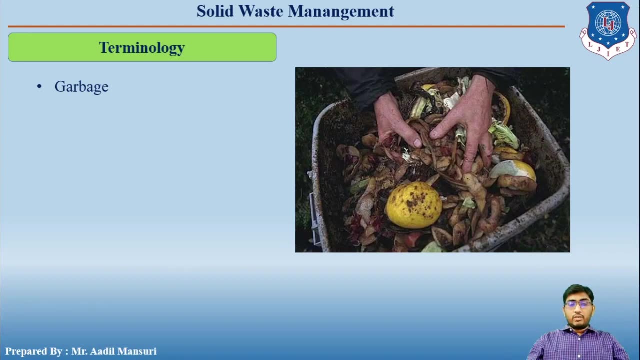 450 to 900. okay, so let us now discuss regarding some terminologies. so the first one is the garbage. okay, so let us now discuss regarding some terminologies. so the first one is the garbage: right kg per meter cube. so let me show you the picture of garbage. okay, so in this it will be. 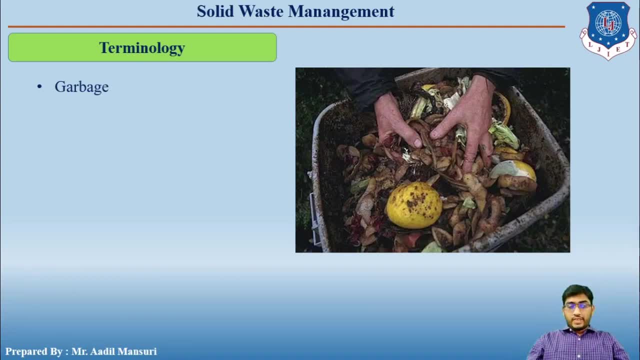 usually the peels of fruits and vegetables or discarded or stale food. right, so all these things are included in garbage. fine, then, talking about rubbish. so rubbish is the combustible or non-combustible solid waste which excludes, which do not include food waste or any other. 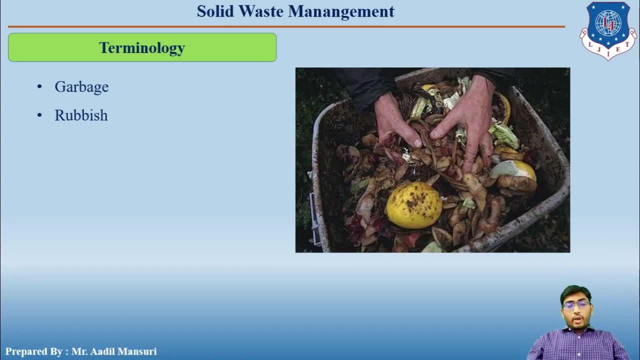 traceable material. okay, talking about typically combustible material. it includes paper, cardboards, plastics, textiles, rubber, leather, wood, furniture and other garden trimmings. okay, talking about non-combustible material, in which included- which are included in rubbish- are glass, crockery, tin cans like pepsi or coca-cola cans. 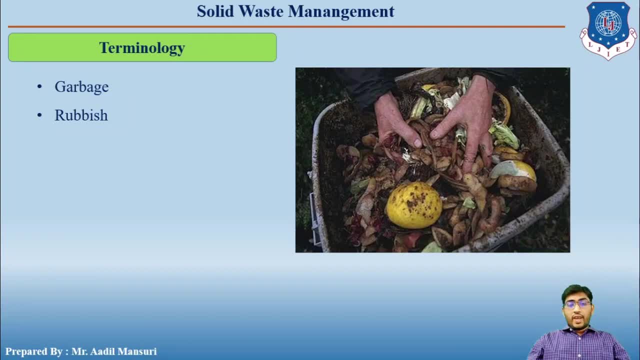 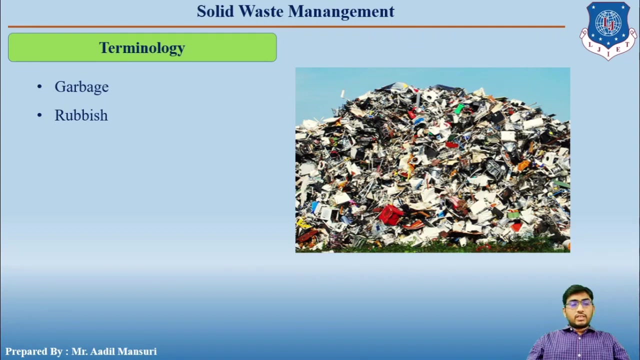 aluminum cans, ferrous and non-ferrous metals, dirts and construction waste. so, talking about its density, it is usually in between 50 to 400 kg per meter cube. okay, so this is the picture of rubbish. let us now talk about ashes and residue, so material which is remaining from burning of wood. 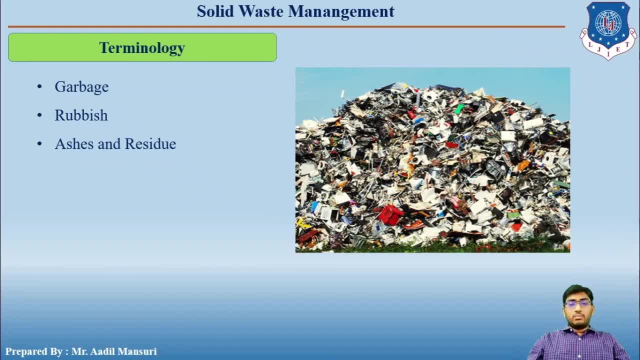 coal, coke and other combustible wastes right are known as ashes, and these are normally composed of fine powdery materials. cinders, clinkers and a of other such materials have been used to condition and small amount of burned and partially burned materials. talking about its, 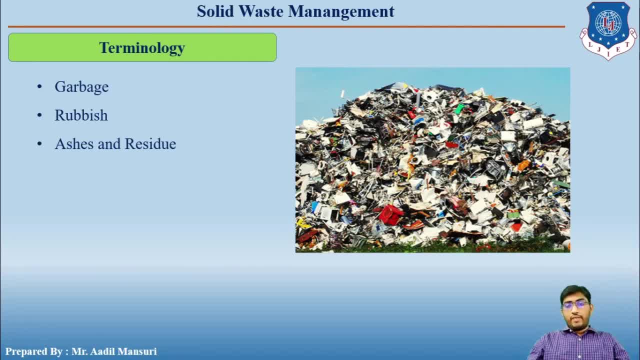 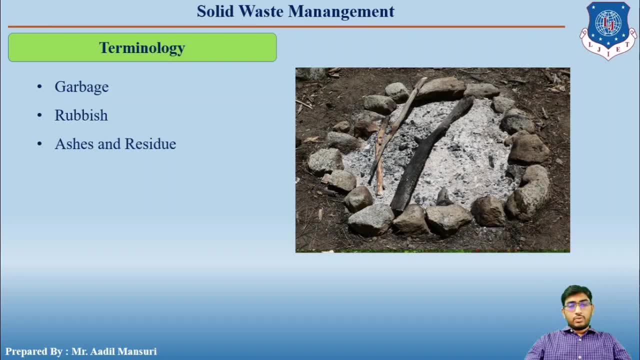 density. it is usually 700 to 850 kg per meter cube. so this is ashes and residue. okay, let's talk about putrefaction. so putrefaction is the process of decay or rotting in a body or other organic matter. okay, then comes the leachate. what? 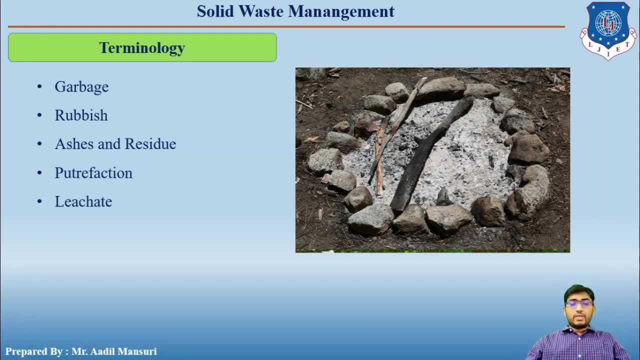 do you mean by leachate? so you might have seen that when there is a stack of this solid waste, some colored liquid, usually black colored liquid, is running out of this stack. okay, so this colored liquid which is coming out of the stack is known as leachate. let me show you the picture. so this is the leachate. 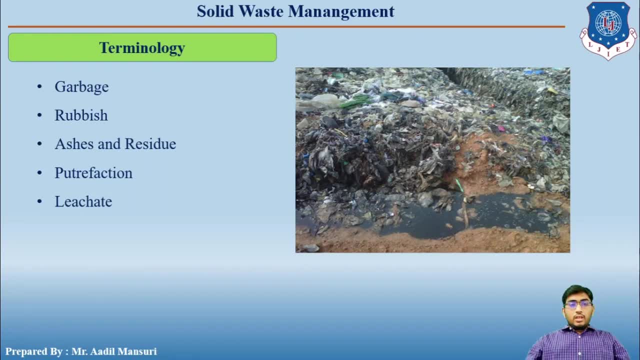 okay, then next is demolition and construction waste. so the waste which are coming out from the buildings or other structures, okay, are classified as demolition waste. right, then, waste from construction or remoulding and preparing of residential or commercial or industrial buildings or other similar structures may include. 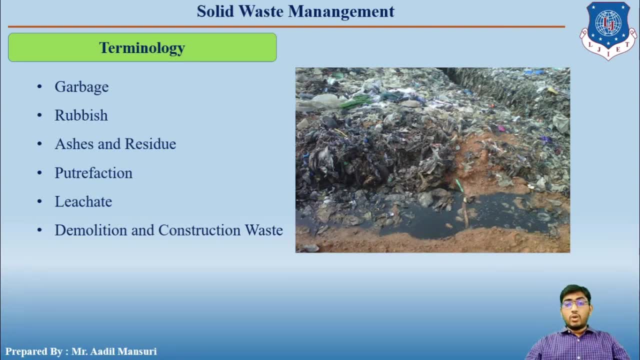 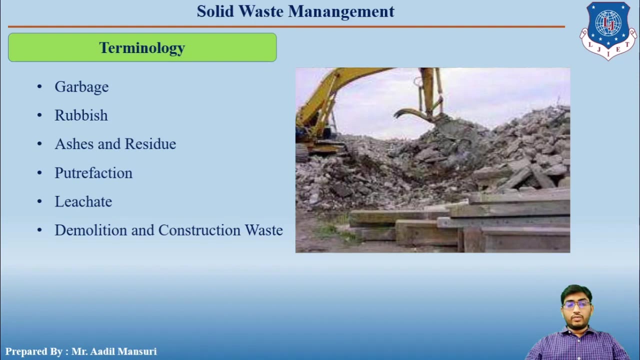 dirt, stones, concrete bricks, right. so these are known as the demolition or construction waste. so this is the picture of debris. okay, then comes special waste. so waste such as street sweeping, roadside litter, catch, brain debris, dead animals, abandoned vehicles are classified as special waste. okay, then, talking about treatment plant waste. so, as we all have created our own, 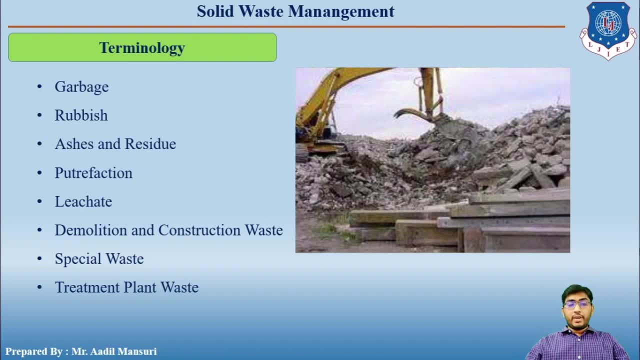 treatment plants. we have natural waste, we have TRH oil and we have Ash and we have brocade as the surfaceût sins all work in bothitto. later then on, the man desires trends of decent treatment plants, and sometimes there is an embroidery, claimed now you kind of double-check and to be treated. well then, one of the things that 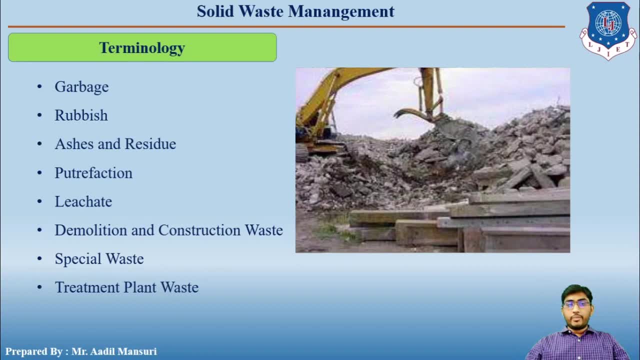 perhaps you can find, is these velocidade xenomer佐уш 영상을. you will see, for the reason why this micro decomp opens. this wo possible in any situation studied regarding water treatment plant and wastewater treatment plant. so, whatever this sludge is there? right, we have to dump on the landfill site. okay, 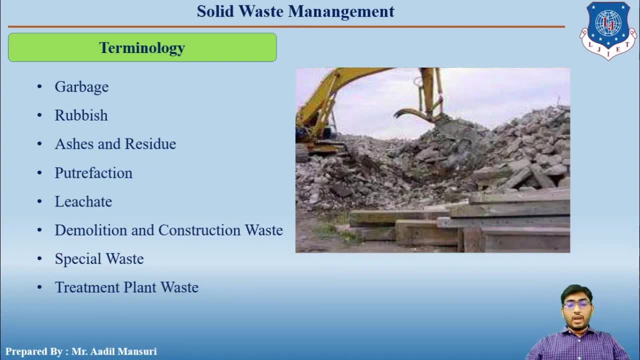 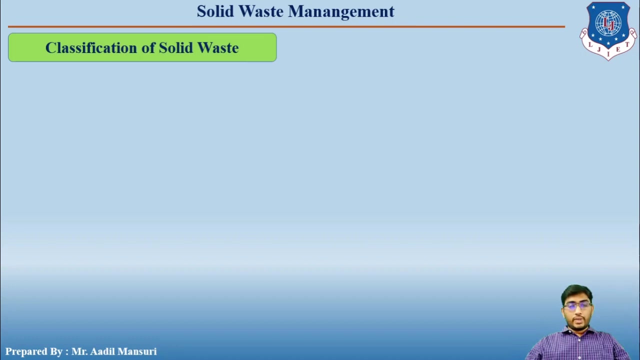 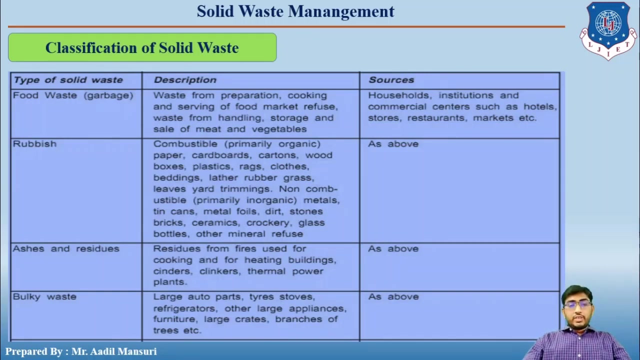 so the solid and the semi-solid waste which are coming out from what water or wastewater or industrial waste treatment facilities are included in treatment plant waste? okay, let us move ahead. so talking about classification of solid waste. so type of solid waste, description and sources. there is a tabular form, okay. 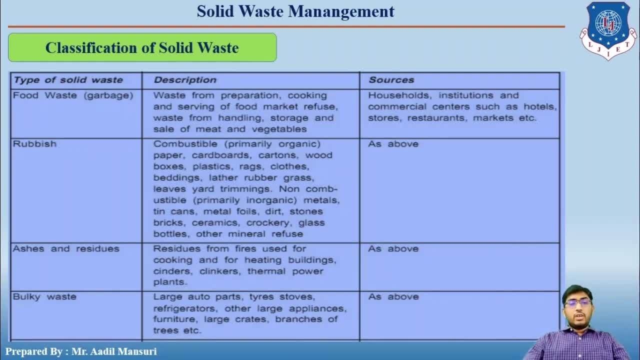 so food waste. that is usually garbage. so the waste from preparation, cooking and serving of food market refuse waste from handling, storage and sale of meat and vegetables are included in food waste. okay, so what are the different sources for this? households, institutions, commercial centers such as hotels, stores, restaurants. 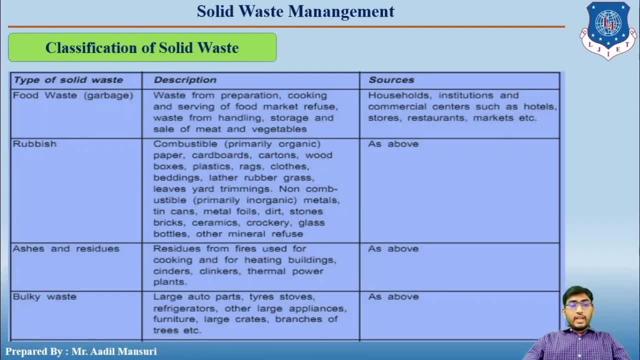 markets, etc. okay then rubbish, combustible material if I talk about, then they are partly sorry. primary organic, okay, paper, cardboard cartons, wood boxes, as discussed earlier. right then non-combustible metals, cans, dirt stones, bricks, etc. okay, sources are remaining the same then: ashes and residue, residue from fires used for cooking and for. 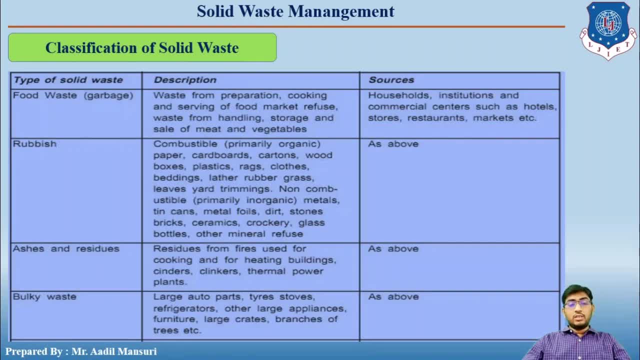 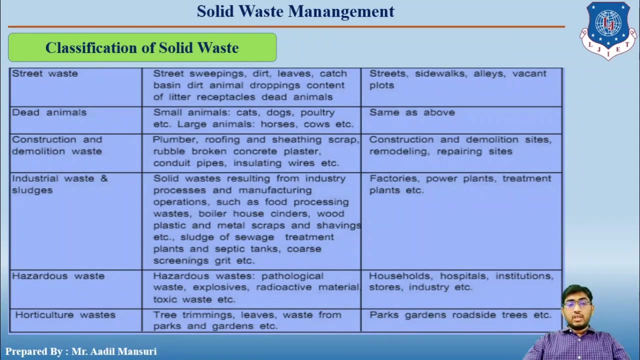 hitting buildings, cinders, clinkers, thermal power plants, etc. food waste was dead animals, okay. here so streets, sidewalks, alleys, wagon plots- are the some of these forces right? so this is the classification of solid waste, right. then comes dead animals, then construction and demolition, industrial waste, hazardous waste and horticulture waste. 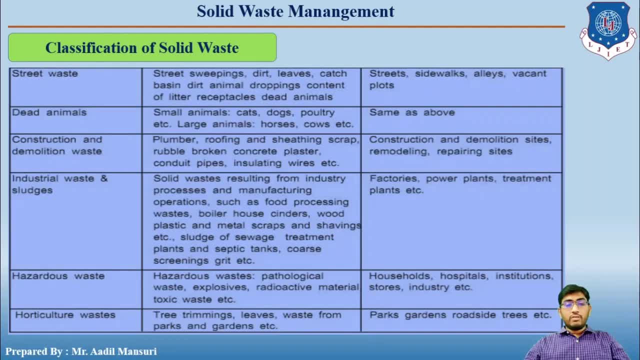 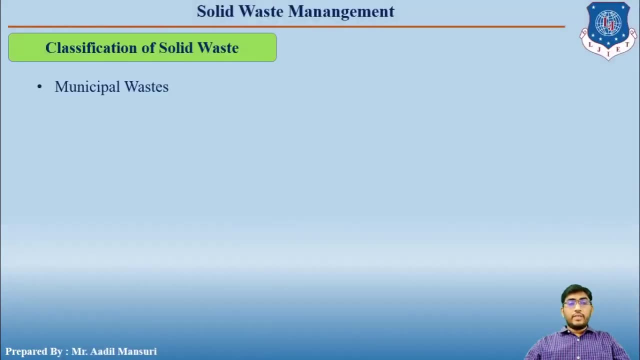 so horticulture waste means tree trimmings, leaves, waste from parks and gardens, right, so where we get from parks, gardens or roadside trees clear. so this was in detail classification. then further solid waste can be classified as municipal waste, then hazardous waste and industrial waste. let us talk about municipal solid waste. okay, so municipal solid waste. 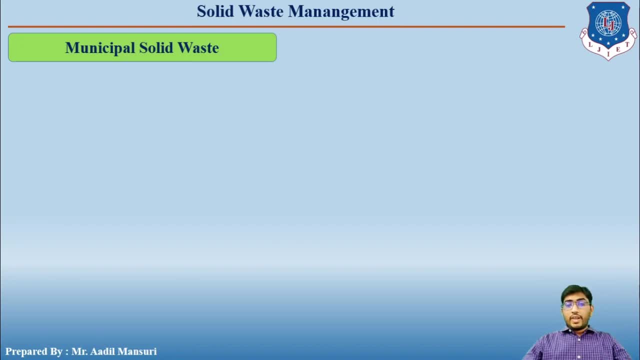 include waste from residential open areas, such as parks, trees- uh sorry, streets, playgrounds, etc. and treatment plants waste, which includes, right then, apart from that, garbage, rubbish, ashes, demolition and construction waste, so all these things are included in solid waste. okay, then, classifying. classifying solid waste. so nine percent. 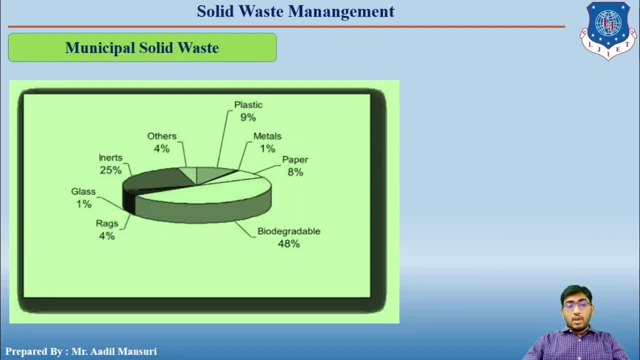 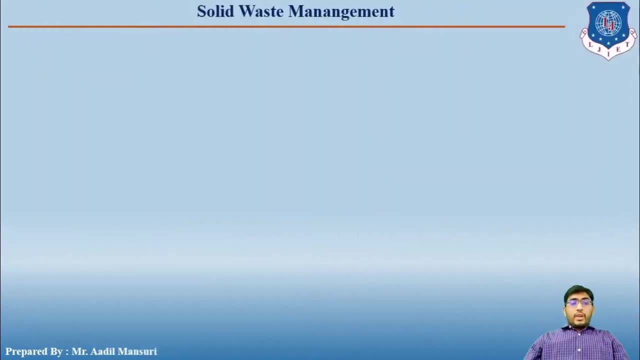 plastic, one percent metal, eight percent paper. forty eight percent are the biodegradable metals. then rags, which includes four percent glass, one percent inert material, twenty five percent, another two percent. okay, so next it is industrial waste. right, so industrial waste are those waste which are arising from industrial activities and typically include rubbish ashes. 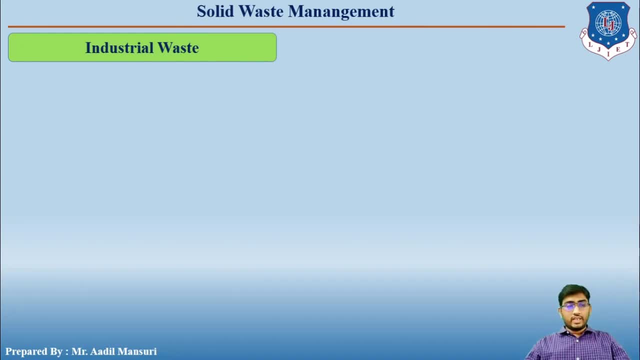 demolition and construction waste, spatial waste and hazardous waste. okay, so you can see the industrial waste picture. further, hazardous waste: so the waste that poses substantial danger, immediately or over a period of time, to either human beings, plants or animal life are classified as hazardous waste. okay, now a waste is classified as hazardous waste. 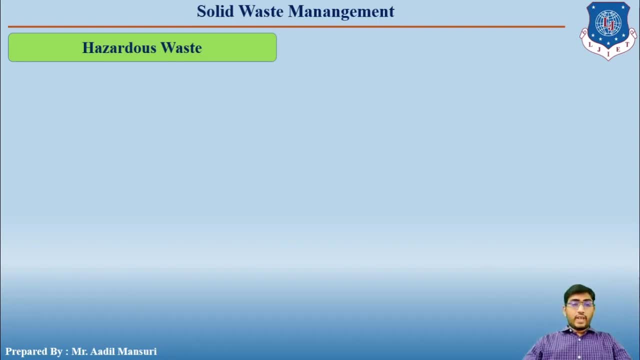 if it exhibits any kind of characteristics like ignitability, corrosivity, reactivity or toxicity. right in the past, hazardous waste were often grouped into following categories: that is, radioactive waste, chemical waste, biological waste and flammable waste and explosives. okay, the chemical category includes waste that are corrosive, reactive or toxic.